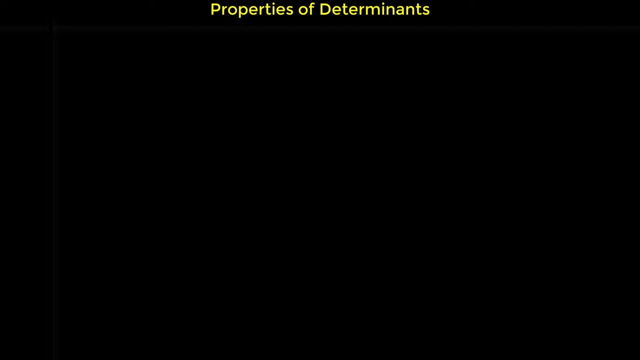 In this video we want to learn some properties of determinants. The first property is that if we have a square matrix, A, and we multiply it by a constant like K, determinant of this new matrix is equal to K to the power of N times by determinant of the original. 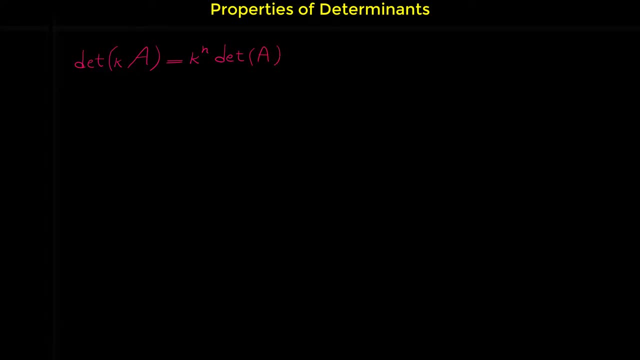 matrix. For example, if we have a square matrix, note that here N is the number of rows or the number of columns of the matrix, because A is a square matrix, so the number of columns is the same as the number of rows. For example, if A is a 3 by 3 matrix and we multiply it by a constant, 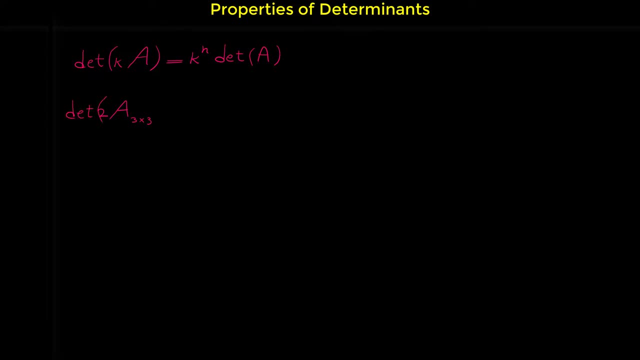 like 2, the determinant of 2A is equal to K to the power of N times. by determinant of 2A We multiply the matrix by a constant, like 2 to the power of 3, to the power of 3, because the matrix 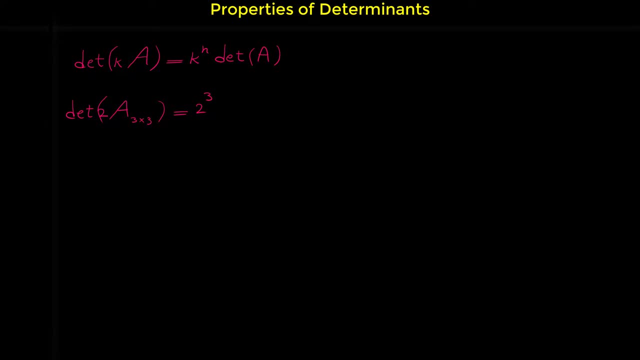 A is 3 by 3.. So determinant of 2A equals 2 to the 3 determinant of A. If the matrix B is 2 by 2 and we multiply it by a constant like 5, the determinant of 5B equals to 5 to the power of 2,. 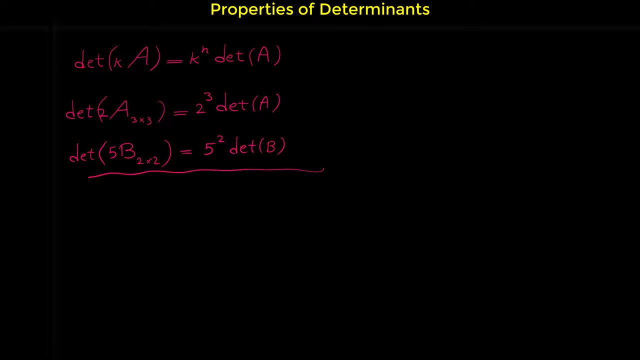 determinant of the matrix B. Now let me show you an example how we can use this property for answering questions. Suppose we have a matrix A in the form of 2, negative 3,, 1,, 5 and the matrix B is equal to. 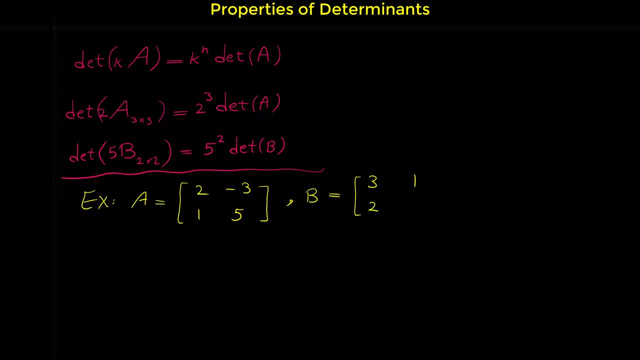 3, 1, 2, 4.. Then we are asked to find determinant of 3, A, B From this property that we learned here. first, we can write this in the form of 3 to the power of 2. 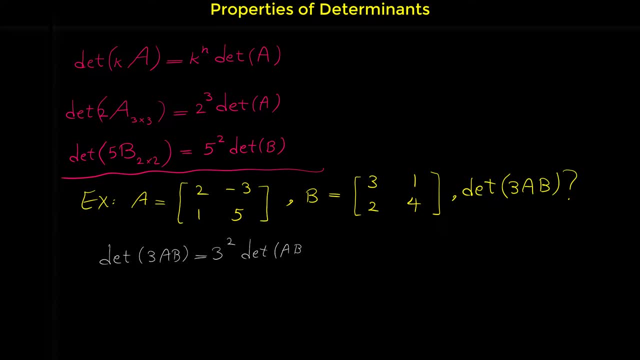 determinant of A. We can bring this constant to the determinant of A And write it as 3 to the power of 2.. Why the power is 2 here? Because the matrix A and B are 2 by 2.. So when we bring this constant, 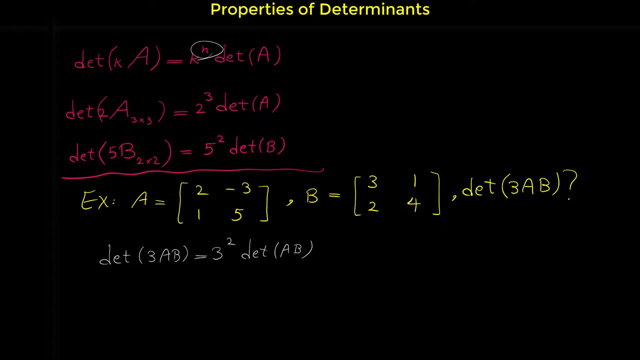 from the determinant, we have to raise it to the power of n, which n is the number of rows or columns. And because these matrices are 2 by 2, so we raise 3 to the power of 2.. Now maybe you think. 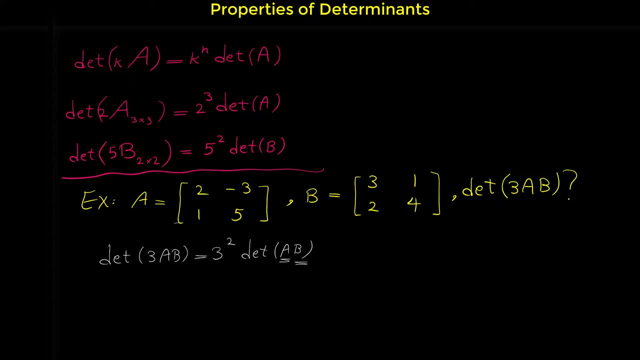 first you have to multiply A by B. Yes, you can do this, Multiply A by B and then find the determinant of the new matrix. But it's a bit hard to multiply this matrix by this matrix. There is an easier way to find. 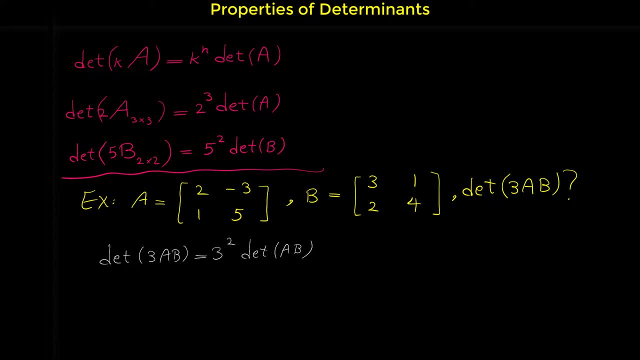 the determinant of A times B. If you remember from the previous video, we learned that determinant of A times B is one of the properties of matrices: multiplication of matrices. Determinant of A- B equals to determinant of A times B. Determinant of B. 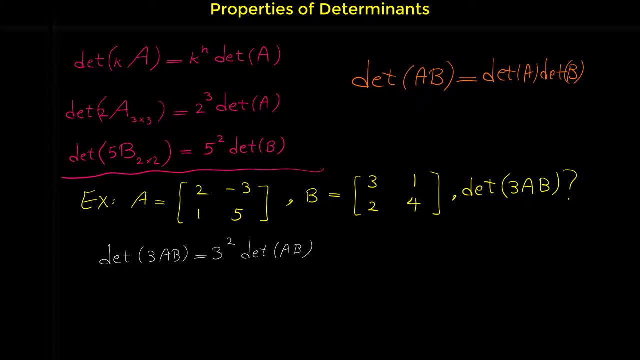 It's easier to use this property for finding determinant of A- B. So instead of multiplying A by B, we can say: this equals to 3 to the 2,, which is 9, times by determinant of A. B based on this property is equal to: 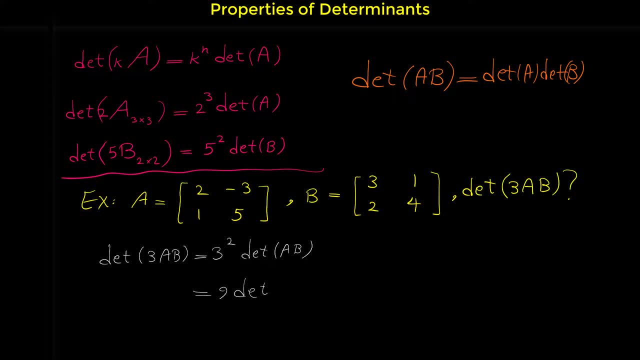 determinant of A times by determinant of B. Determinant of the matrix A is 2 times 5, which is 15, 10, sorry- minus negative 3 times 1.. 10 minus negative 3 is 13.. So this equals 9 times 13 times 1.. 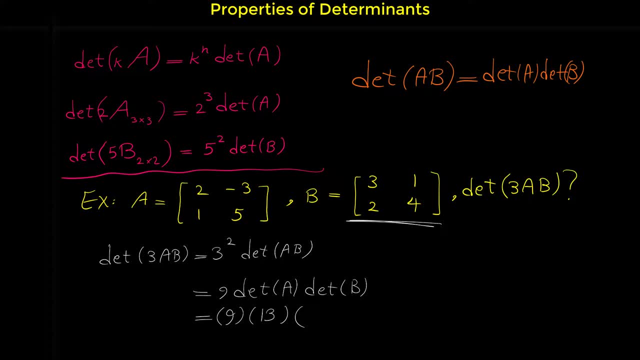 Determinant of the matrix B is 12 minus 2, 10.. Now, 9 times 13 is 173.. And 10 times 13 is 117.. 117 times 10 is 1170.. Let me show you another example. 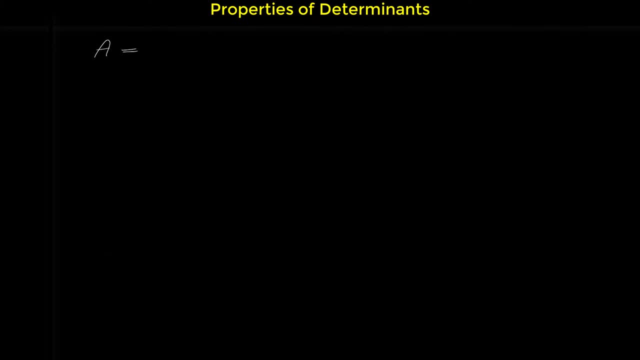 Suppose matrix A is negative: 1,, 2,, 5,, 0,, 1,, 2,, 0,, 0,, 3.. And matrix B is 2,, 1,, 7,, 7,, 5.. 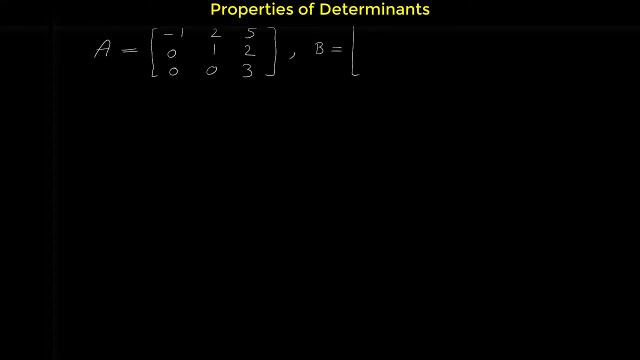 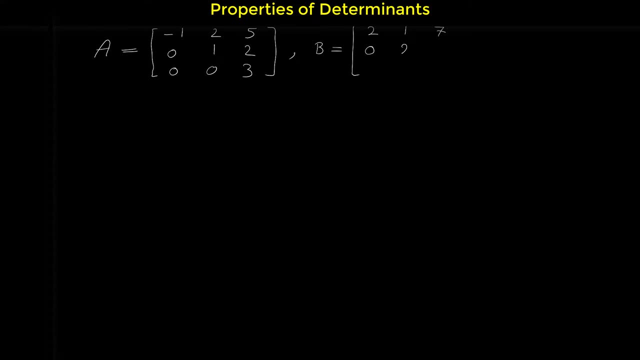 zero two one zero zero, negative one, and we are asked to find determinants of negative three, a, B, a transpose from the above property. we learned that we can bring this out from the determinant because these two matrices are three by three. so when we bring negative three out from the determinant we have to 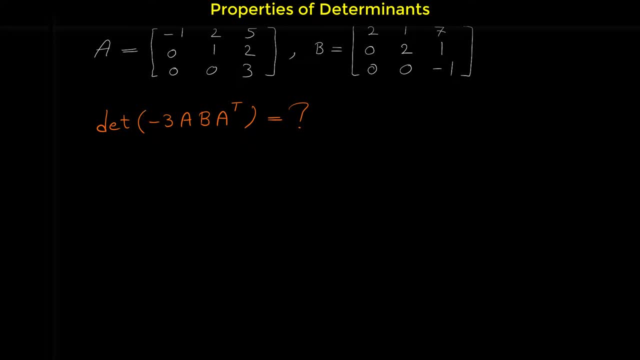 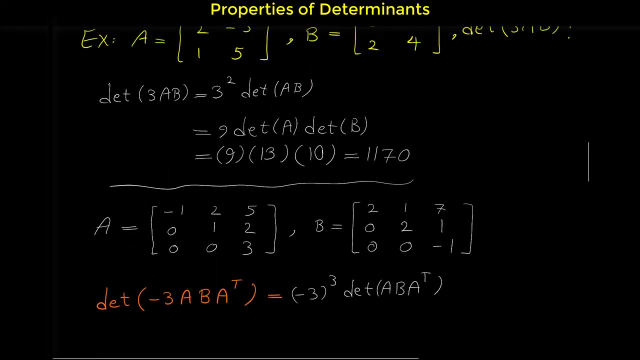 raise it to the power of three. so the first thing that we do here we write this as negative three to the power of three. determinant of a, B, a- transpose. now for finding determinant of a times B times a- transpose again. we use these properties whenever we multiply two matrices by: 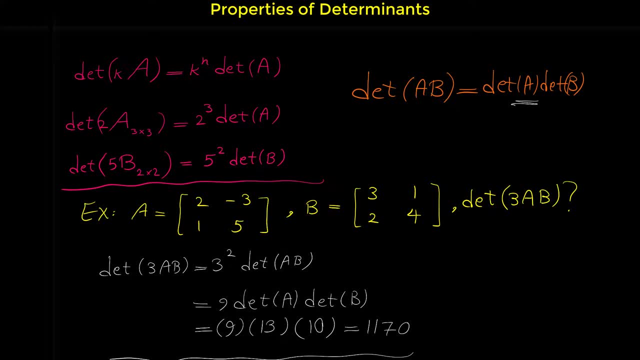 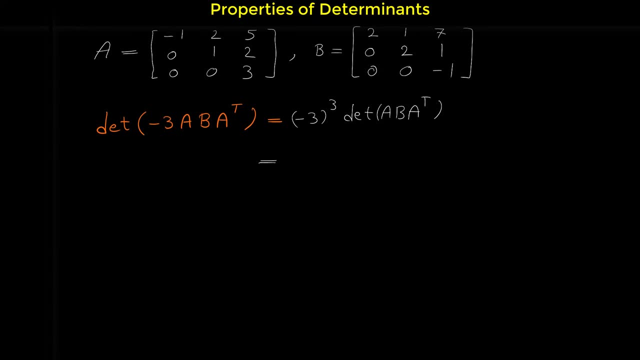 each other. determinant of a times B equals the terminal of the first matrix times the terminal of the other matrix. if we use this property here, we can write this as negative three to the three is negative 27. determinant of a, b, a transpose is determinant of a times by determinant of b times by determinant of a. 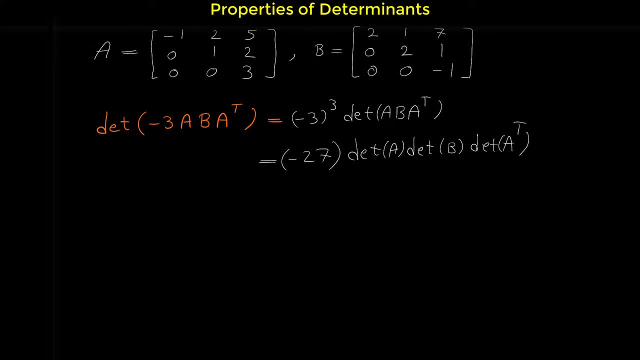 transpose. this is much easier to use this property than multiplying these matrices by each other. if you want to multiply matrix a by b, because these are three by three matrices, it needs lots of calculations. now you have to find determinant of a, determinant of b and determinant of a transpose. 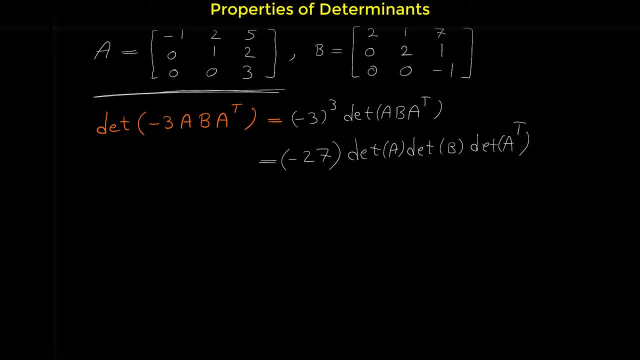 what is the determinant of this matrix? note that this matrix, here its matrix a, is upper triangular. if you are not familiar with triangular matrices, you can watch my videos about triangular matrices and other type of matrices. this is upper triangular matrices because matrix, because all the terms below the diagonal, this is the diagonal of this matrix all. 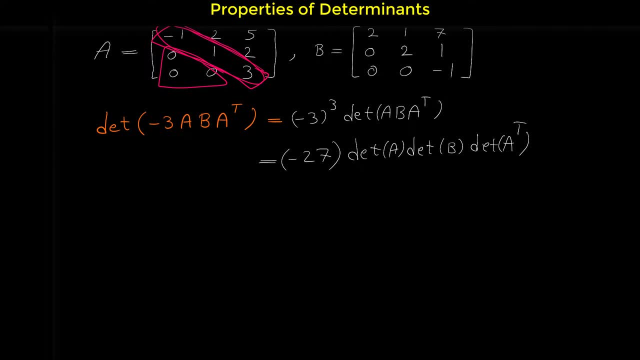 the terms below the diagonal are zeros. so this is upper triangular matrix and when we have upper triangular matrix, determinant is the product of the elements of the diagonal. we know this from the previous video. so determinant of the matrix a is equal to- let's write negative 27 again. determinant of the matrix a is negative 1 times 1 times 3. 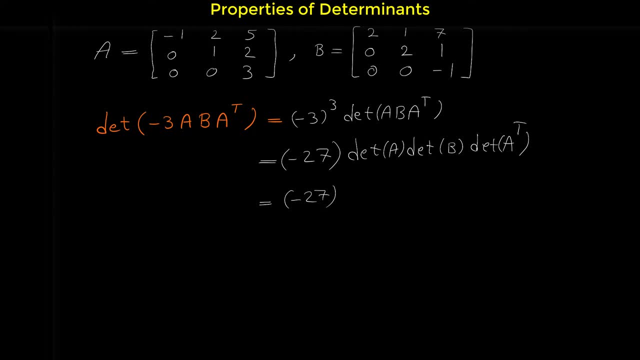 negative 1 times 1 is negative 1 times 3 is negative 3. so determinant of the matrix a is negative 3. determinant of the matrix b, similarly, is 2 times 2 times negative 1 negative 4. again. why we can find determinant of the matrix b in this way? because this matrix is upper triangular. but 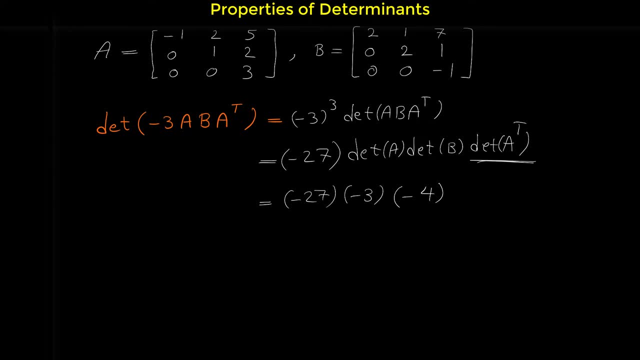 how we can find the determinant of the matrix- a transpose again from the previous video. if you remember, the determinant of the transpose of a matrix is equal to the determinant of that matrix. there is no difference between the determinant of transpose of a matrix and the terminal of the. 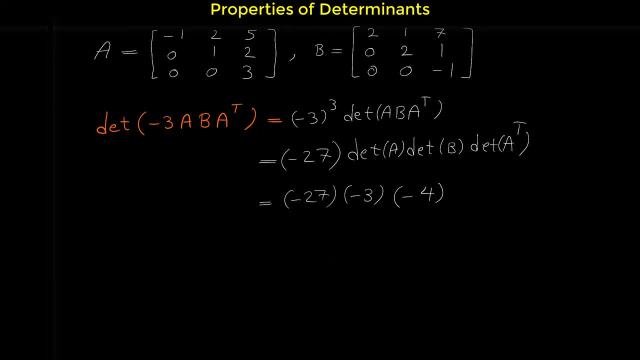 original matrix. so because the terminal of the matrix a is negative 3, so the terminal of a transpose is also negative 3.. now if we multiply these numbers by each other, note that we have four negative, so it becomes positive number. 27 times 3 is 81. 81 times 4 is: 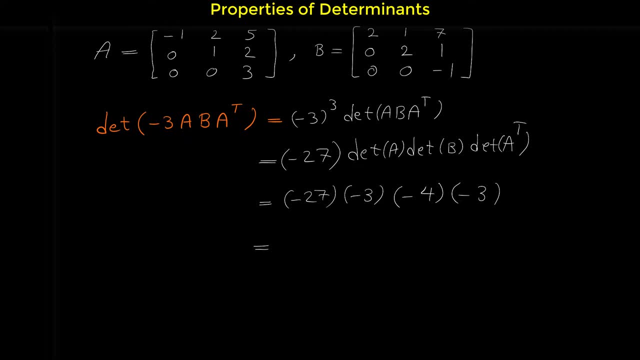 324, and 324 times 3 is 972.. if we have a matrix a and we raise it to a power, say n, note that n is an integer number. two, three: any positive integer determinant of the a to the power of n equals to determinant of the matrix a to the power. 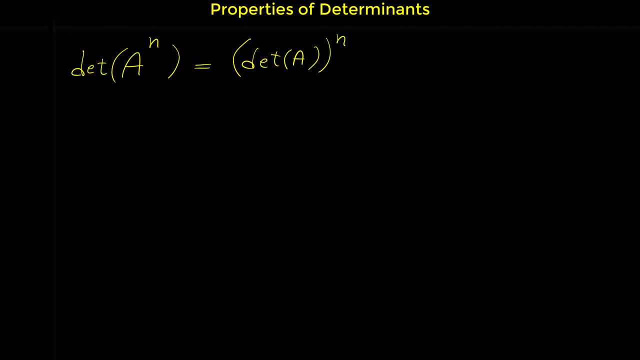 of n, so you can bring n out of the determinant and put it above the determinant if you don't know what is a to the n. for example, if you have a to the 3, a to the 3 means that multiply a by itself three times. 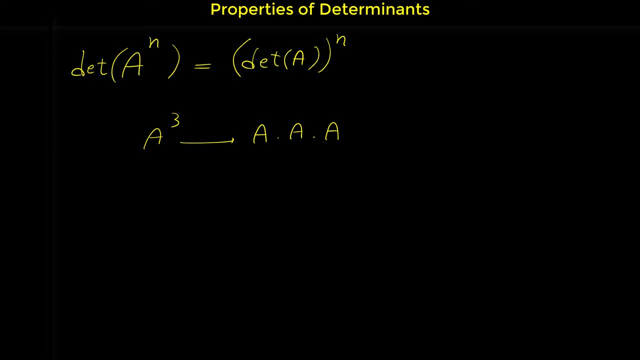 the power of a matrix means to multiply by itself, like the normal power for a number. this property is also one of the useful properties of determinants, because it simplifies answering questions like this. we are given this matrix a equals negative two, three, one, five, and we are 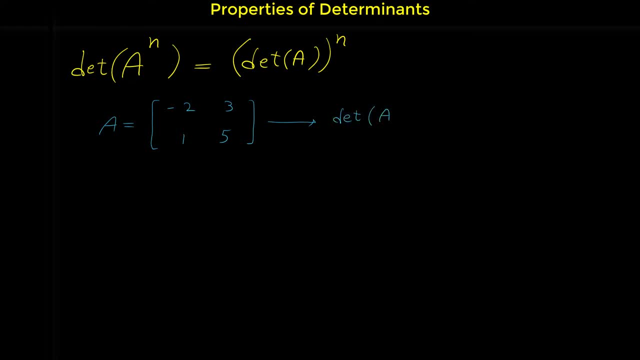 asked to find determinant of a to the power of, for example, a to the three. one way to find this is to multiply this matrix by itself three times and then find the determinant of that. but multiplying a matrix by itself, and multiplying matrices, as you know, it's a bit hard and needs some. 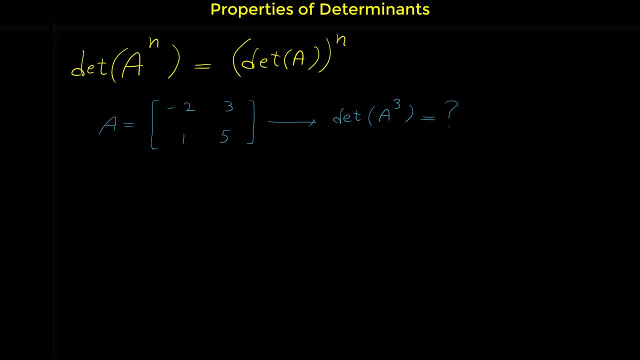 calculations. it's possible to make mistakes during those calculations, so it's better to use this relation that we learned here. we know that if we want to find the determinant of a to the three, say this is equal to the determinant of a. then raise it to the 3.. what is the determinant of? 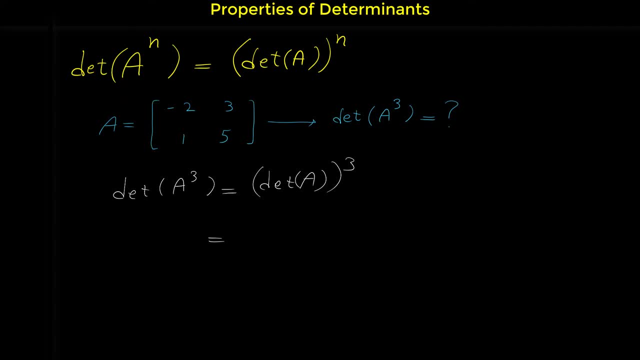 this matrix: negative 2 times 5 is negative. 10 negative 10 minus 3 is negative 13.. so now we have to raise negative 13 to the power of 3, because the power is negative. sorry, because the power is odd. the power is 3 negative remains. now we have to multiply 13 by itself. 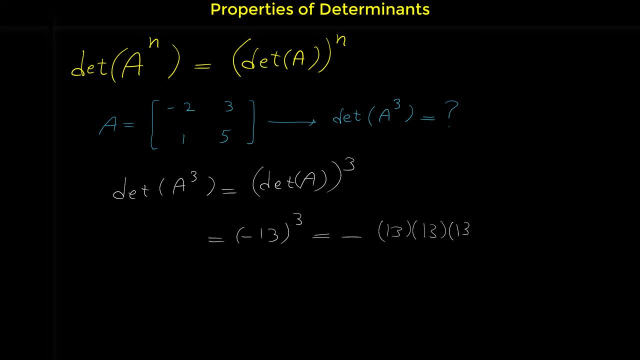 so 13 times 13, 3 times 30, is 2197. let me show you one more example. the matrix a is negative: 1, 2, 3, 1. matrix b is 2, 4, 1, 1, and we want to find determinants of: 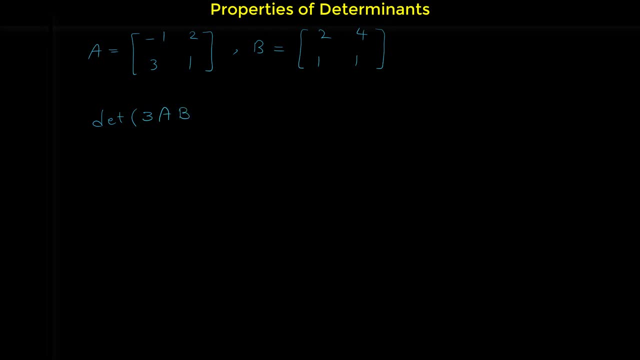 3 a b square. first note that we can bring 3 out from the determinant and raise it to the power of 2, y to the power of 2, because these matrices are two by two. then we have determinant of a- b square. now note that three to the two is nine and determinant of a times b square is determinant. 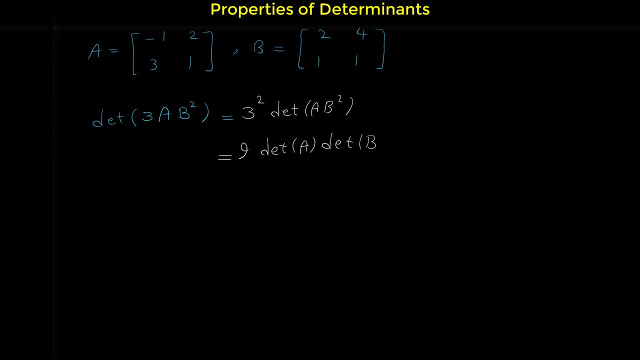 of a times the determinant of b squared. when we have the product of two matrices determinants of the product equals the terminal of the first one times the determinant of the other one. the matrix a is negative one times one is negative one two times three is six negative one minus two. 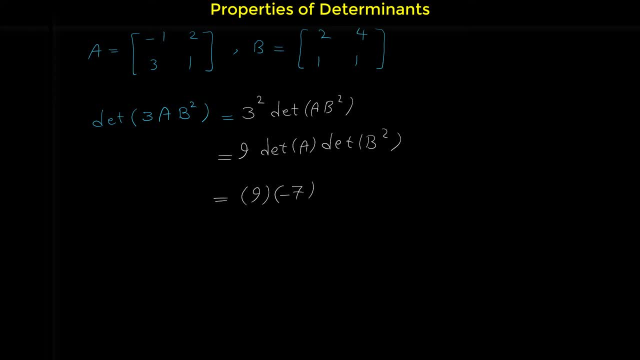 times three is minus seven. so the terminal of the matrix a is negative seven. if you don't know how to find the determinant of matrices two by two, three by three, watch my video about the terminal of matrix. finding the terminal of matrix. the terminal of b squared is determinant of b. 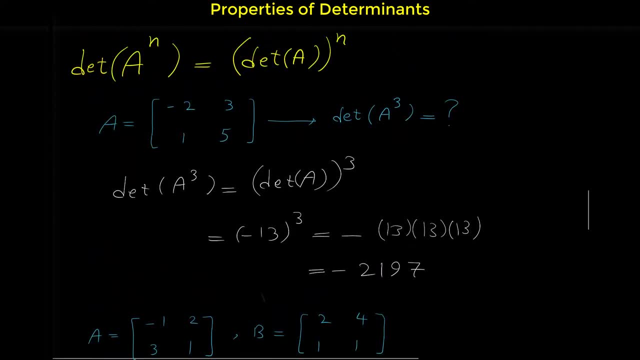 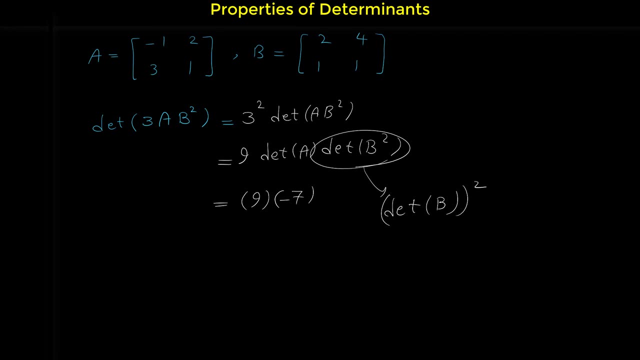 squared. as we learned here, you can use this property. so the terminal of b square is the terminal of b to the power of two. what is the terminal of this matrix? two times one, two minus four, negative two. now, if we raise negative two to the power of two, equals four. so times by four, nine times negative seven is. 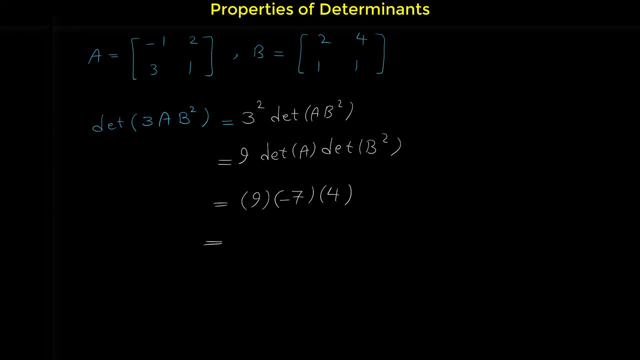 negative sixty three. negative sixty three times four is negative 252.. let me show you one more property of determinant of matrices, and then i finish this video. suppose we have m by n matrix a. so for that matrix a is not a square matrix. and we have another matrix, say b, which is n by m. 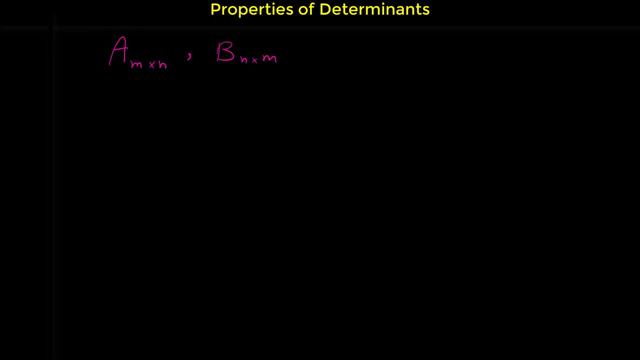 so none of these matrices are a square. but if your attention a times, b is a square matrix because when we multiply a by b, the result is a matrix, is a new matrix which is m by b. why? because the first matrix is m has m rows. so the result of multiplying a by b has animals and the matrix b. 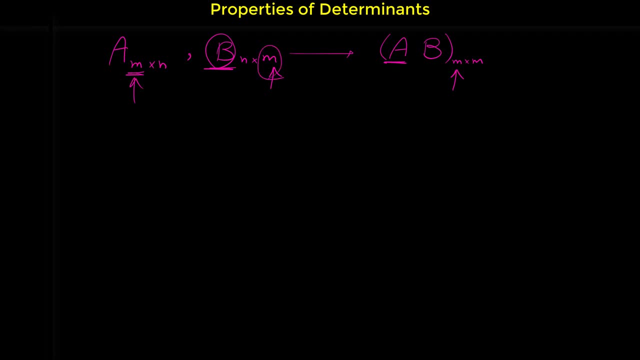 has n m columns, so the product of them has m columns. so when we multiply a by b, we get m by m matrix. this is a square matrix. now note that if it is important, if m be greater than n, then determinant of this new matrix, determinant of a times b determinant. 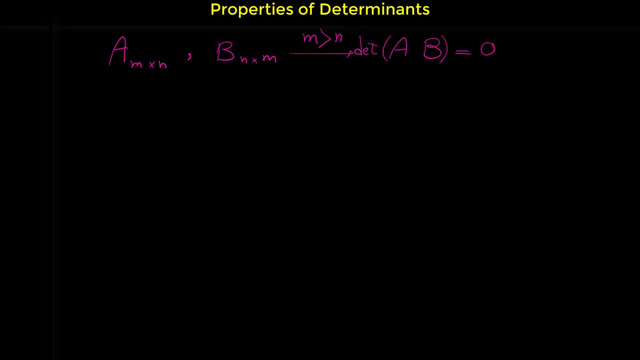 of a times b is zero, you don't need to calculate determinant of a times b, it's always zero. this is one of the properties determinant of matrix. for example, suppose you have matrix a which is, say, four by three, and the matrix b is three by four, so that a the size of rows of a the first. 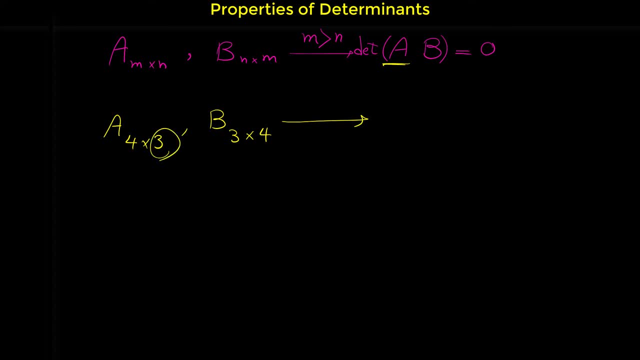 one is greater than the number of columns, it's important that m should be greater than n. if we multiply a by b, the result is a four by four matrix. determinant of this matrix is zero. you don't need to calculate and it doesn't matter. what is matrix a? what is matrix always? 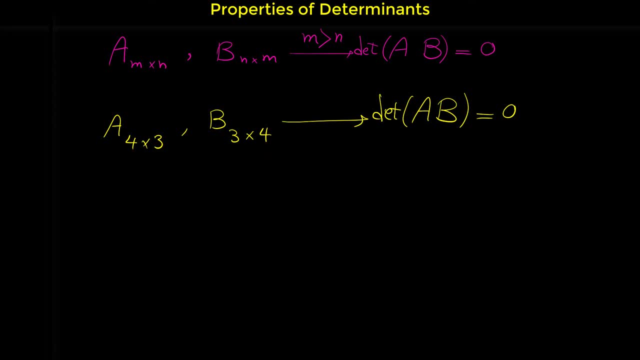 the determinant of a times v is zero. but note that determinant of b times a is not necessarily zero, because b times a is three by three. determinant of the bigger one, bigger matrix, is zero, because a times v is four by four, but b times a is three by three, so only a times.